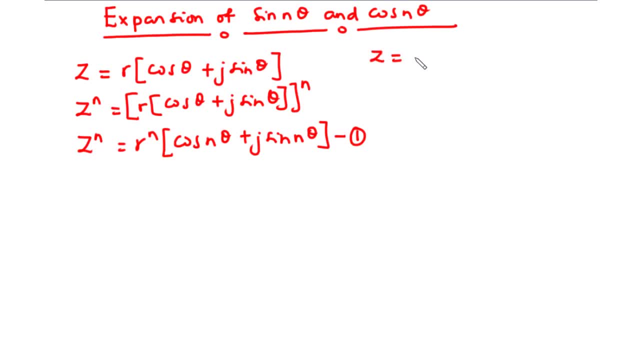 in the exponential form as z equals r times e exponent j theta, So z exponent n equal to r times e exponent j theta, all exponent n, and this becomes r exponent n times e exponent j theta n. now let's call this equation two, so it is reasonable to conclude that cos theta. 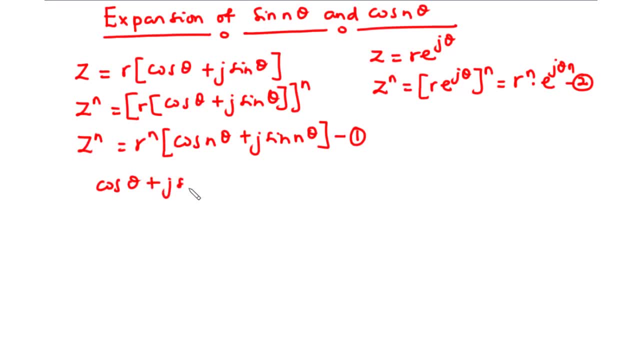 plus j sine theta, all exponent n is equal to cos n. theta plus j sine n theta, and that is also equal to e exponent j theta n. so for instance, if n is equal to two and then we say that cos theta plus j sine theta, all exponent two is equal to cos two, theta plus j sine. 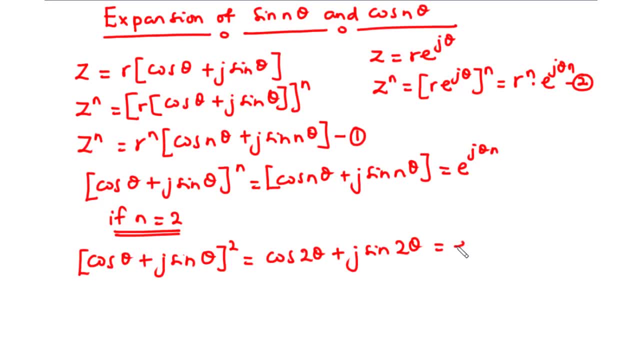 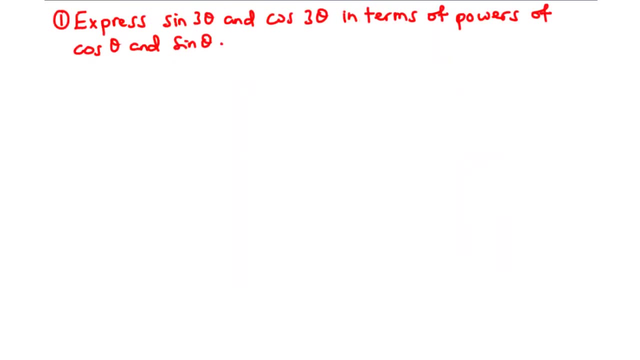 two theta, and that is also equal to e exponent- two j theta. so, having this in mind, let's try some examples. so, for example, one express sine three theta and cos three theta in terms of powers of cos theta and sine theta. now let's try this example. 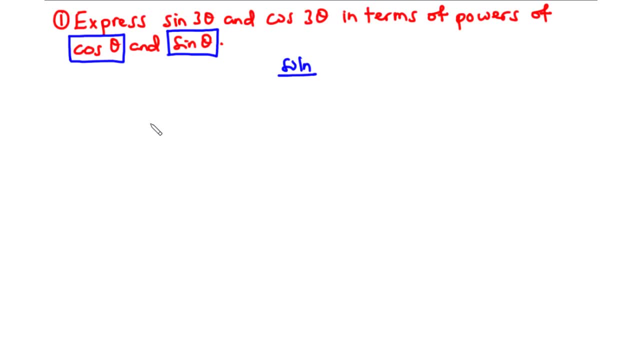 so according to the Morvius theorem we know that cos n theta plus j sine n theta is equal to cos theta plus j sine theta, all exponent n. so from this we can say that cos three theta plus j sine three theta is equal to cos theta plus j sine theta all exponent n. 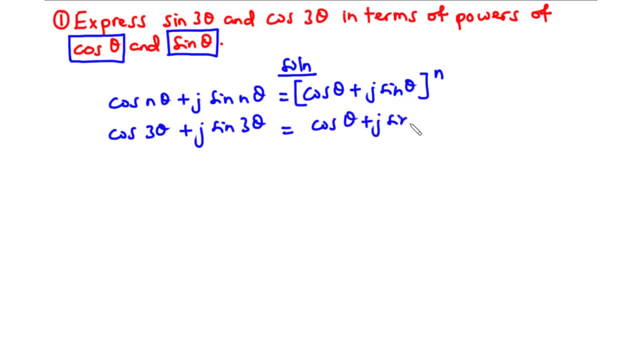 so from this we can say that cos three theta plus j sine three theta is equal to cos theta plus j sine theta, all exponent n, all exponent 3.. So how do we expand cos theta plus j sine theta? r cube, Now we know from the 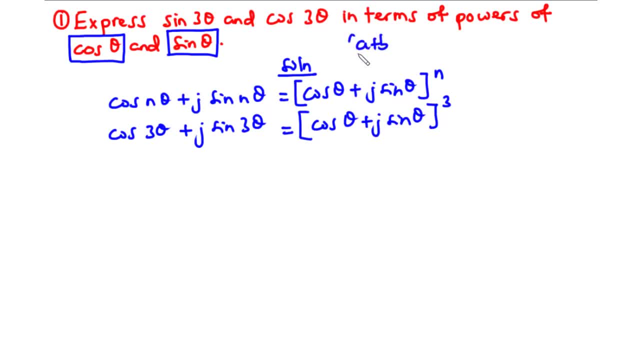 expansion of a plus b r cube that this expression is equal to a cube plus 3a square times b plus 3a times b square plus b cube. So basically we are going to use this to expand cos theta plus j sine theta r cube. Therefore we have cos 3 theta plus j sine 3 theta equals. we have a to b. 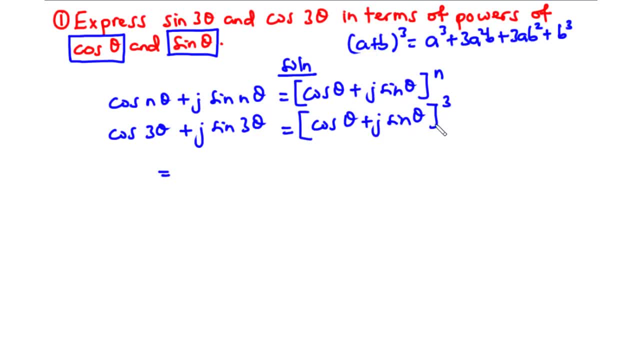 cos theta and then b to b j sine theta. So we have a cube, so that becomes cos cube. theta plus 3 times a square, So that becomes cos square theta times b, which is j sine theta plus 3 times a. We have a to b cos theta and then b to b j sine theta, So this becomes j square. 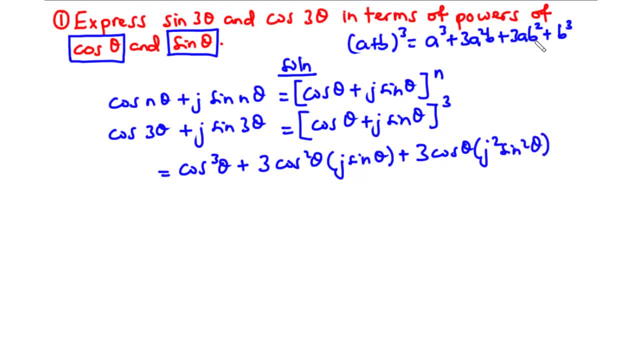 sine square theta, because we have b square plus b cube, So that becomes j cube times sine cube theta. Now let's simplify further. So we have cos cube theta plus 3 times j, So this becomes 3j cos square theta sine theta. Here we have j square to be negative 1.. So this: 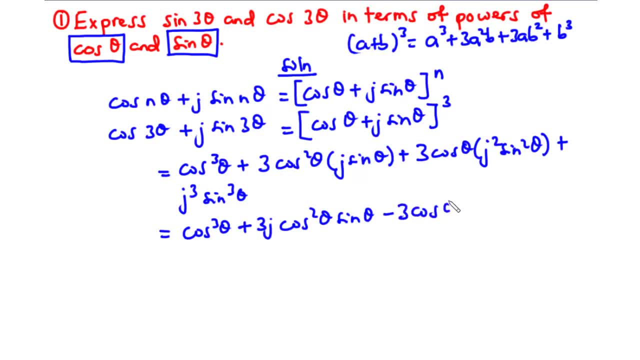 becomes negative 3. cos theta sine square theta. And then we have j cube. Now j cube is equal to negative j. So this becomes negative j sine cube theta. Now let's group the individual terms into real and imaginary components. So we have cos 3. 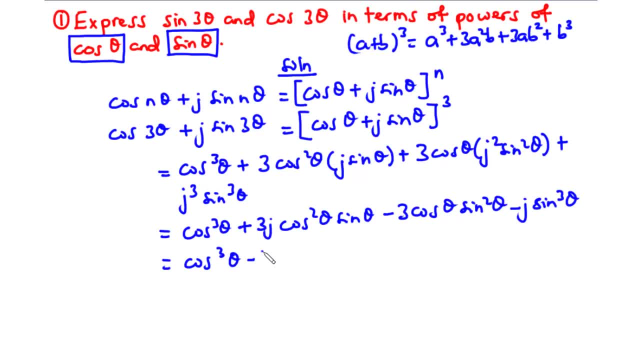 theta minus 3 cos theta sine square theta. Now that's 3 cos theta sine square theta. So this is for the real part, and then for the imaginary we can factor out j and then inside of the bracket we have 3 cos square theta. 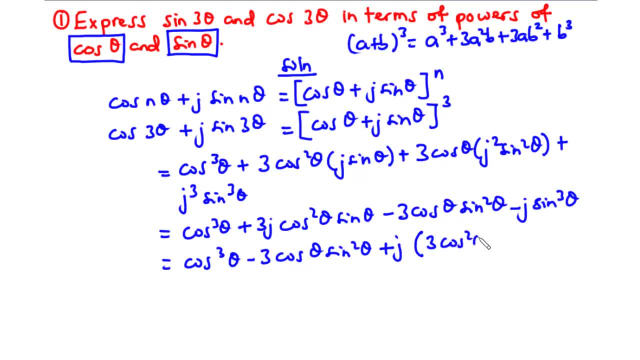 sine theta. So 3 cos square theta sine theta minus sine cube theta. So we have this to be the real part and then this to be the imaginary part. Now, from the onset we know that 3 cos theta sine square theta step will leave as negative 3 cos square theta sine theta. And if we ultimately calculate점 factor of the instead of sin2sqt, and the Joo tip burner simplifies it, then we end up to d. This gives us h cos 3 theta sine square theta, 2 ihm3sqt minus sine 3 cos square theta sine theta minus sine qt theta. 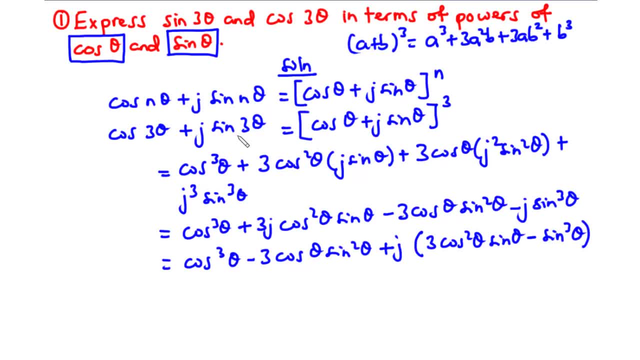 Eternal rest of the full sum. cos3θ is the real part and then jsin3θ is the imaginary part. Therefore, cos3θ is equal to cos3θ minus 3cosθ- sin2θ. Now, from the question we are asked to express sin3θ and cos3θ in terms of powers of cosθ. 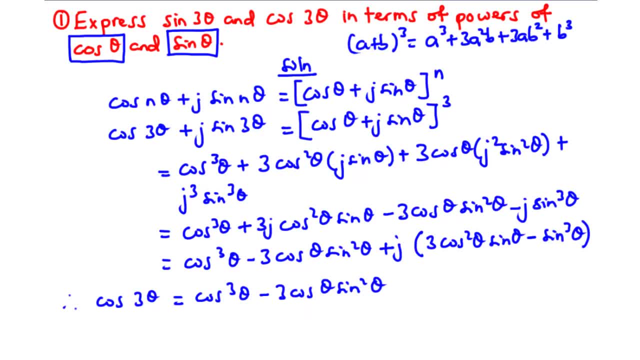 and sinθ. So for the real part, we are going to express that in terms of powers of cosθ, and also for the imaginary part, we are going to express in terms of powers of sinθ. So we need to express sin2θ in terms of powers of cosθ. 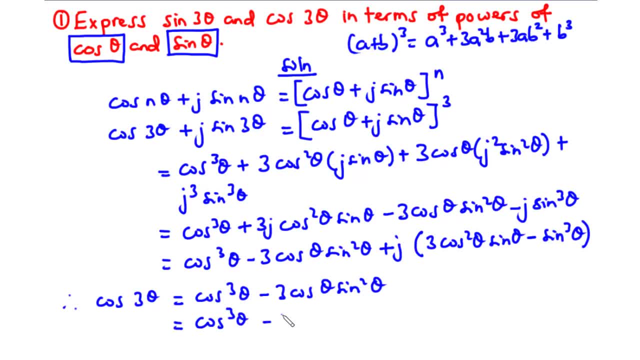 So we have cos3θ minus 3cosθ. Now we know that sin2θ plus sin2θ, Sin2θ plus cos2θ is equal to 1.. Therefore, sin2θ is equal to 1 minus cos2θ. 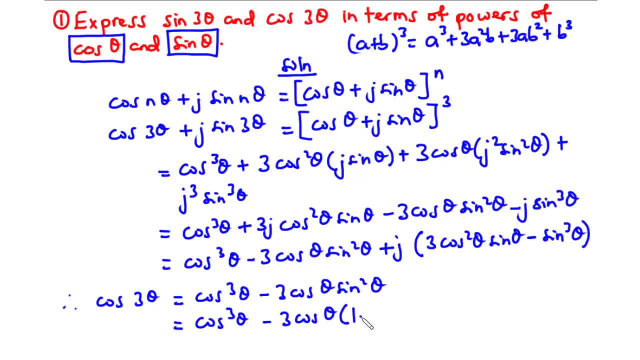 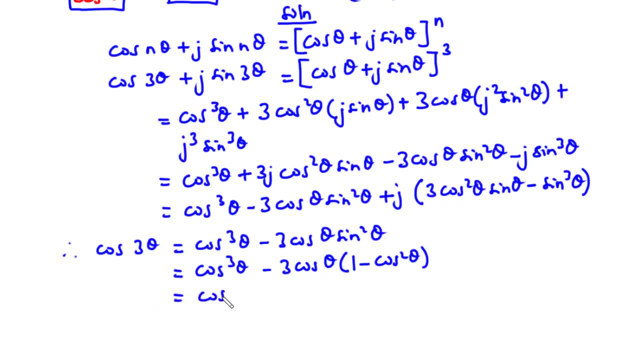 So instead of writing sin2θ, we are going to write 1 minus cos2θ. Now let's simplify further. So this becomes cos3θ minus. we have negative 3cosθ times 1.. So that becomes negative 3cosθ minus sin2θ. 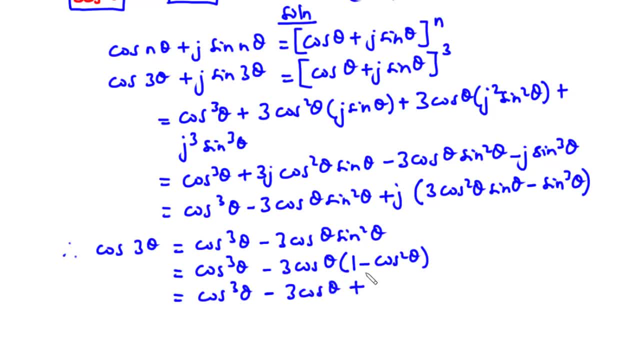 And then we have negative 3cosθ times, negative cos2θ, So that becomes positive 3cos3θ. Now we have cos3θ, we have 3cos3θ, So we can add the two so that we have 4cos3θ minus 3cosθ. 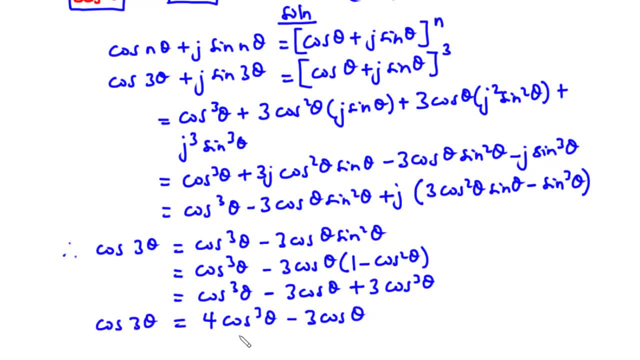 Therefore we say that cos3θ is equal to 1.. So we can add the two so that we have 4cos3θ minus 3cosθ. Therefore we say that cos3θ is equal to 1.. Therefore we say that sin3θ is equal to 1.. 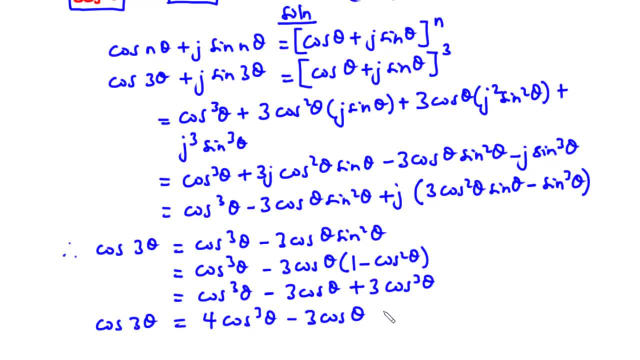 Therefore, we say that cos3θ is equal to 1.. Therefore, we say that cos3θ is equal to 1.. Therefore, we say that sin3θ is equal to 1.. Therefore, we say that 4cos3θ minus 3cosθ. 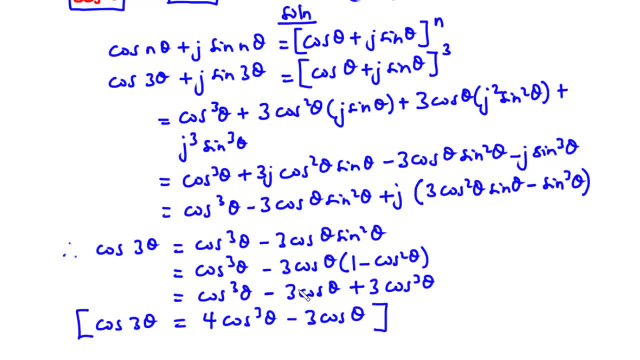 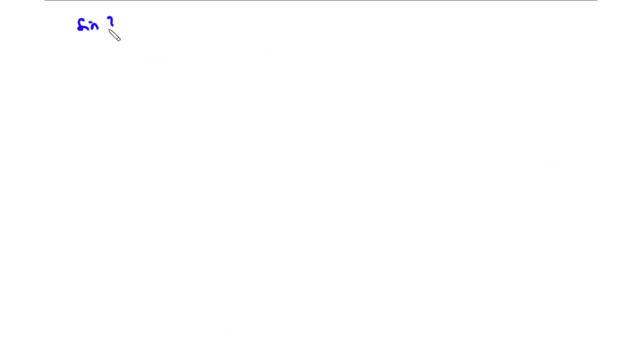 Now let's move on to sin3θ. So for the imaginary part we have: sin3θ equals 3cos2θ, sinθ minus sin3θ. Now we need to express this in terms of program of powers of sine theta. So we need to change cos square theta to powers of sine theta. 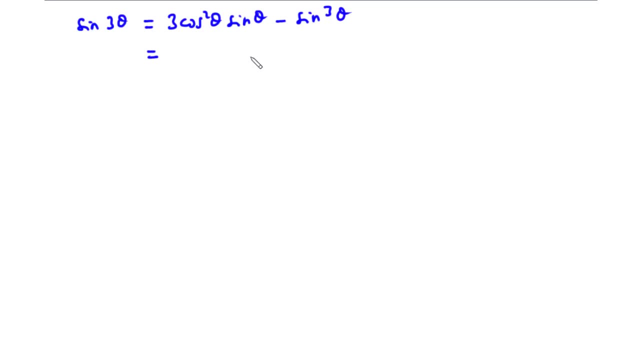 Now we know that sine square theta plus cos square theta is equal to 1.. Therefore, cos square theta is equal to 1 minus sine square theta. So we have 3 times 1 minus sine square theta, times sine theta minus sine cube theta, So we have 3 times 1 times sine theta That. 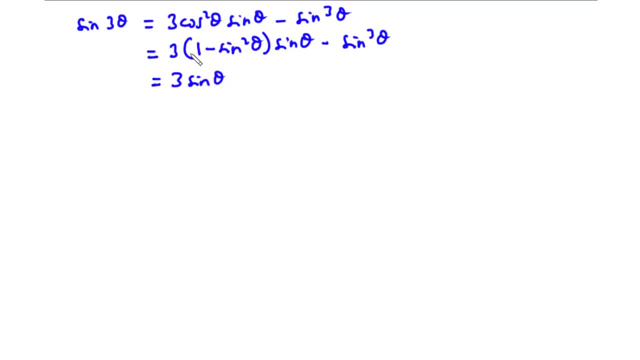 becomes 3 sine theta. And then we have 3 times sine theta, times negative sine square theta, So that becomes negative. 3 sine cube theta minus sine cube theta Negative. 3 sine cube theta minus sine cube theta becomes negative. 4 sine cube theta. 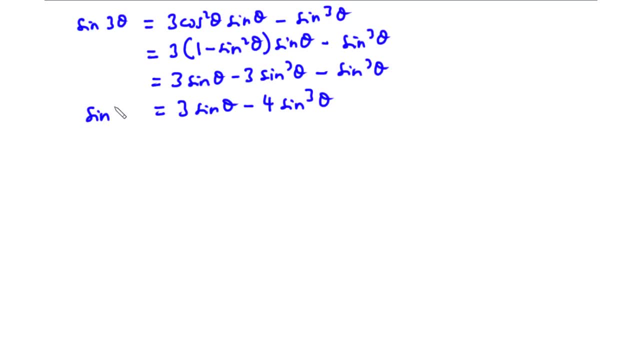 And that is equal to sine 3 theta. Now let's move on to the next example. So for example 2, use the Moivre's theorem with n equals 4 to prove that cos square theta is equal to 1 minus sine square theta. 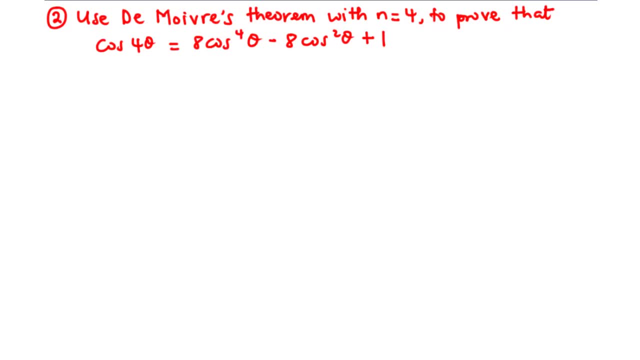 Plus 4 theta is equal to 8, cos exponent 4 theta minus 8. cos square theta plus 1.. So from the Moivre's theorem we know that cos n theta plus j sine n theta is equal to cos theta plus j sine theta, all exponent 4.. 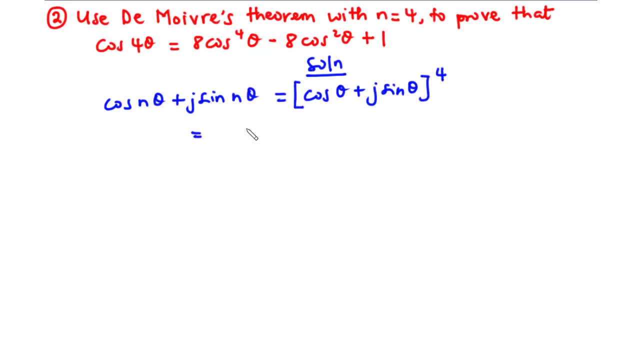 Now let's expand the expression we have on the right hand side. So the expansion of a plus b exponent 4 is equal to a exponent 4 plus 4 times a exponent 3 times b plus 6 times a exponent 2 times b square plus A player times a square double. 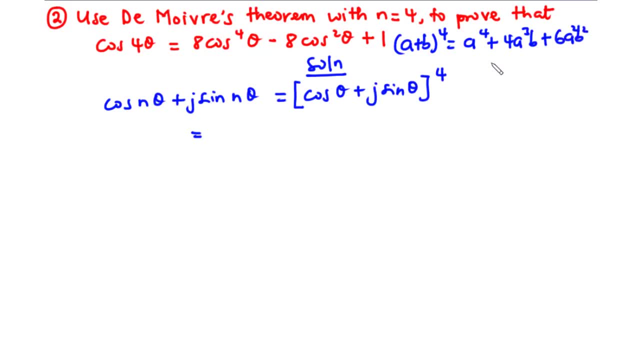 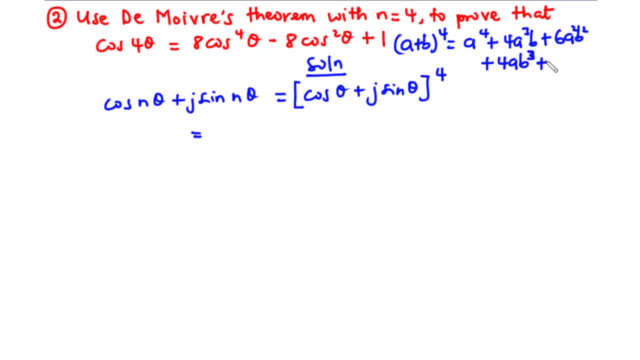 Bye, Bye. b cube plus b exponent 4. so we are going to use this to expand cos theta plus j sine theta, all exponent 4. so we have a to b cos theta, we have b to b j sine theta. now let's do the expansion. 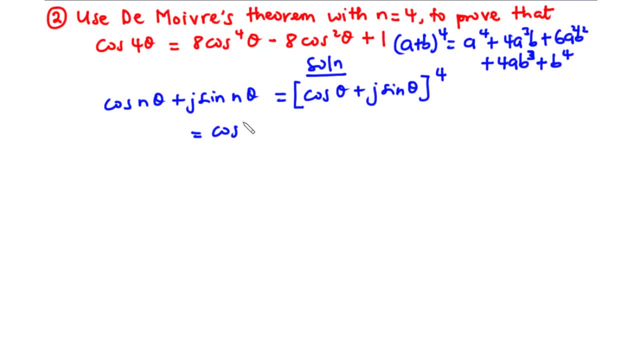 so a exponent 4 becomes cos 4 theta plus 4 times cos cube theta times j sine theta plus 6 cos square theta times j square sine square theta plus 4 cos theta times j cube sine cube theta plus b. exponent 4 is j exponent 4 sine 4 theta. 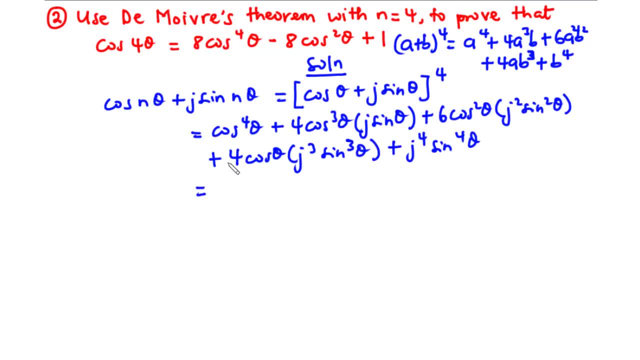 now let's simplify further. so this becomes cos 4 theta plus we have 4 times j, so that is 4 j cos cube theta sine j, sine theta. now this time we have j square, so j square becomes negative 1, so this becomes minus 6. 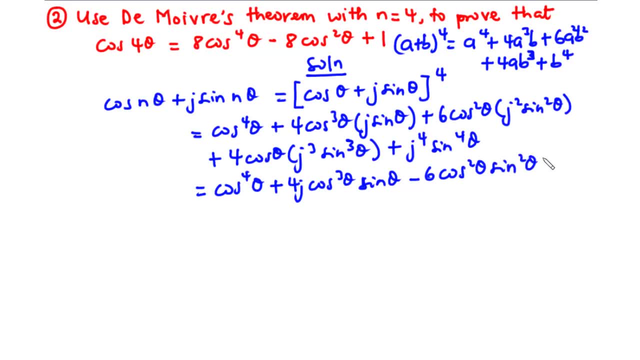 cos square theta, sin square theta. then we move on to: we have j exponent 3, which is negative j, so that becomes minus j. we have wake 4 cos theta sine cube theta. j exponent 4 is 1, so 1 times sine 4 theta becomes sine 4 theta. 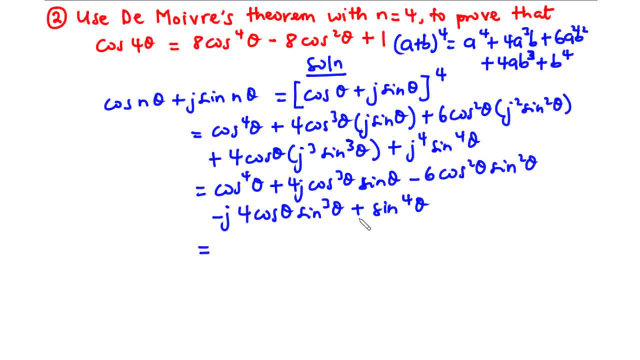 now let's group the terms into real and imaginary components. so for the real part we have cos 4 theta minus 6 cos square theta, sine square theta and then plus sine 4 theta. this is for the real part, and then for the imaginary we have j into bracket. we have 4 cos cube theta, sine theta. 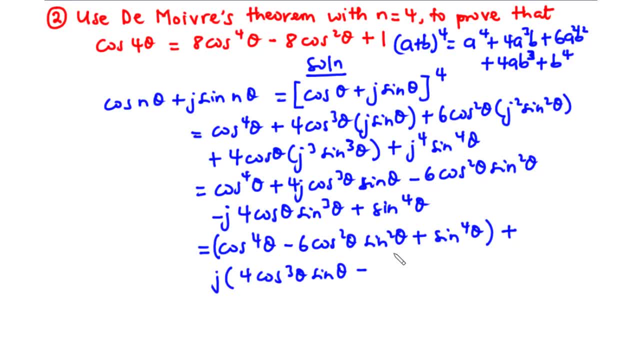 minus 4 cos theta sine cube theta. so we have this as the real part and also the imaginary part. now we know that cos 4 theta is the real part. therefore cos 4 theta is equal to cos exponent 4 theta minus 6 cos squared theta. 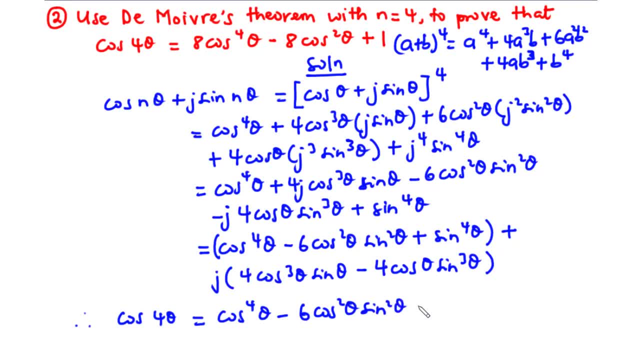 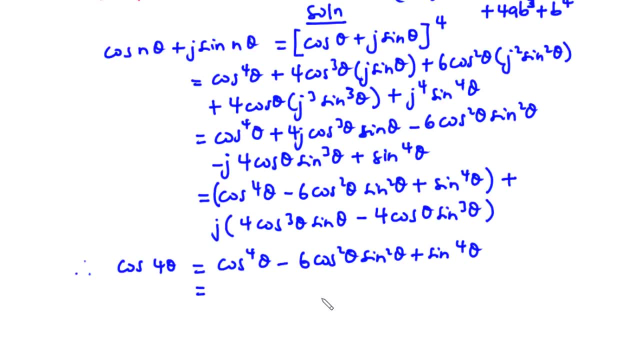 sine 4 theta, sine cube theta. so we have this as the real part and also the imaginary part sine square theta plus sine exponent 4 theta. so we can replace sine square theta with 1 minus cos square theta, so this becomes cos exponent 4 theta minus 6 cos square theta times 1 minus cos square theta. 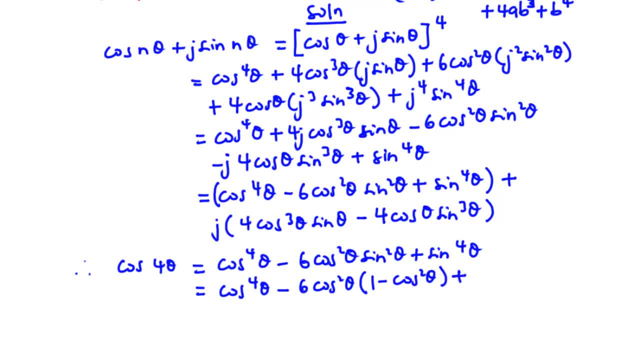 plus, now sine exponent 4 theta can be simplified as sine square theta times sine square theta, so that also becomes 1 minus cos square theta times 1 minus cos square theta. so we can simplify this as cos exponent 4 theta minus negative 6 cos square theta times 1 is negative 6 cos square theta. 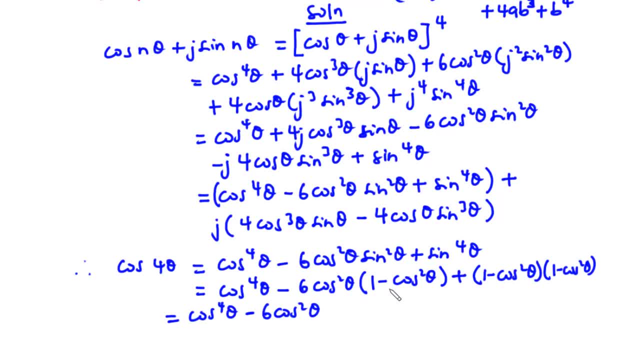 And then negative 6 cos square theta. times negative cos square theta becomes plus 6 cos exponent 4 theta Plus. here we have 1 times 1, which is 1.. We have 1 times negative cos square theta, which is negative cos square theta. 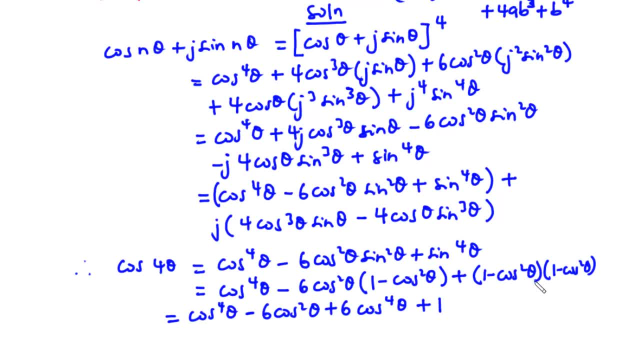 we also have 1 times negative cos square theta. So this becomes negative 2 cos square theta and then negative cos square theta. times negative cos square theta becomes plus cos exponent 4 theta. Therefore we have cos exponent 4 theta plus 6 cos exponent 4 theta.